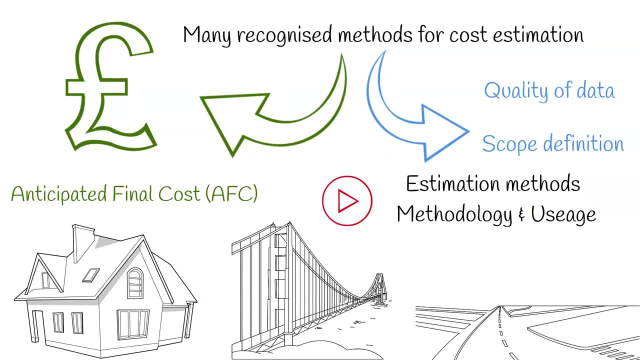 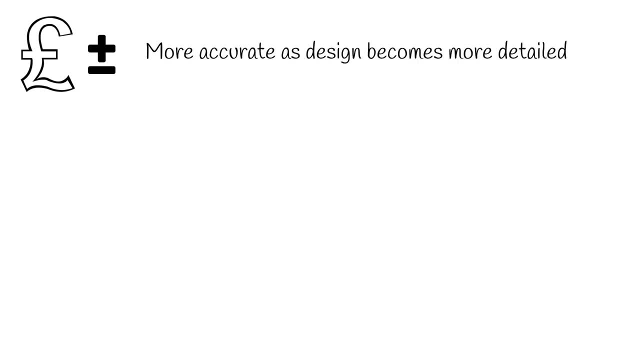 available, how they work and when they should be used. As you would expect, the estimated cost for a project becomes more accurate as design becomes more detailed and, as a result, the chosen method will likely change as a project evolves. The scale and complexity of a project will also affect the 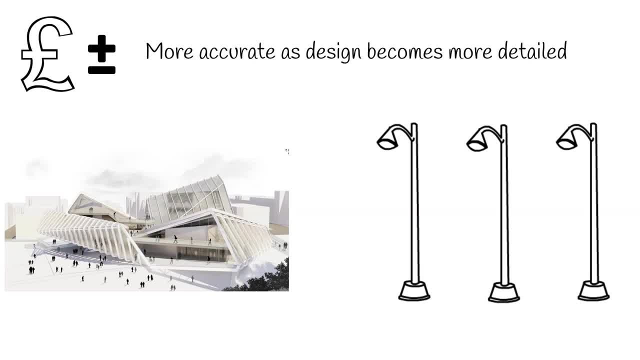 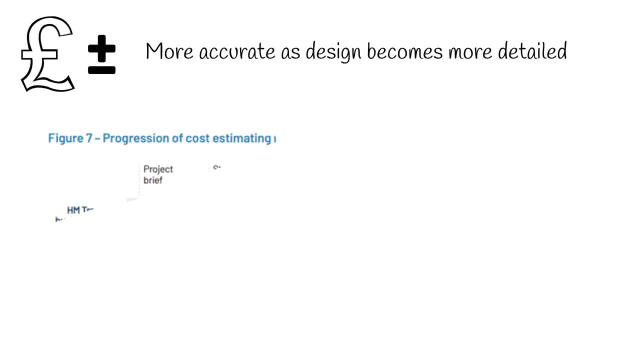 quality of cost data available. Repeatable projects will have more reliable benchmarks and consequences. The estimated cost of a project will also affect the quality of cost data available. This figure, produced by the Infrastructure Projects Authority, shows how the estimation method may evolve as the project progresses. Project estimating can be split into two camps. 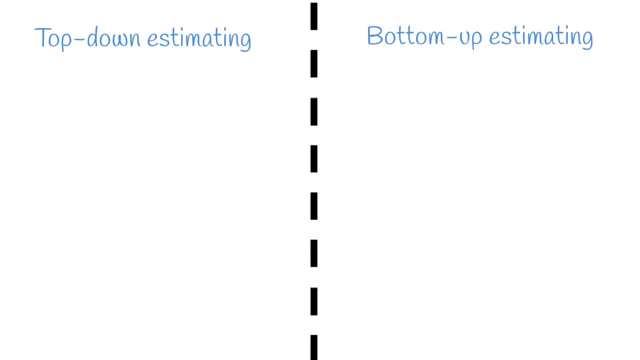 top-down estimating and bottom-up estimating. Top-down estimating is the fastest route for cost estimation. However, it is also considered the most unreliable. It utilizes benchmarking against other projects to form a cost estimate. A top-down approach is often used in very early. 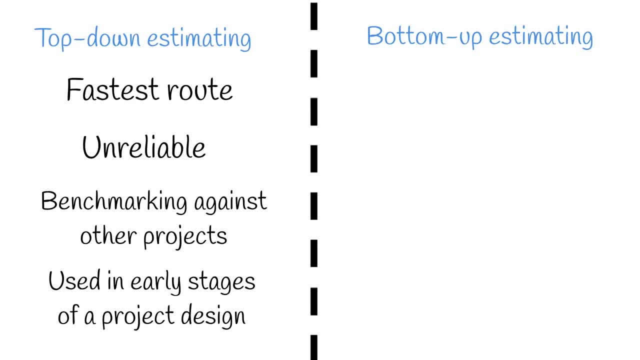 stages of a project and provides as a tool for early decision making. Bottom-up estimating is much more time-consuming. It's based on first principles and provides an accurate cost of a project by understanding the specific task requirements and program duration. A bottom-up 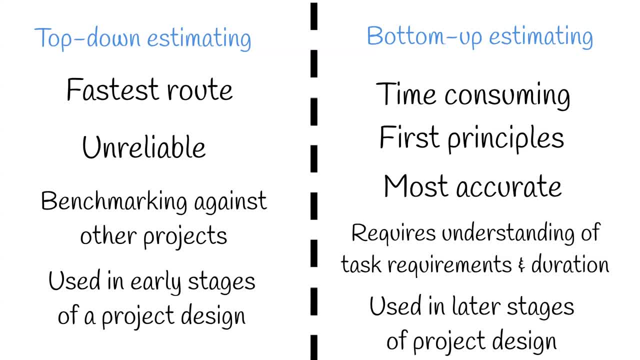 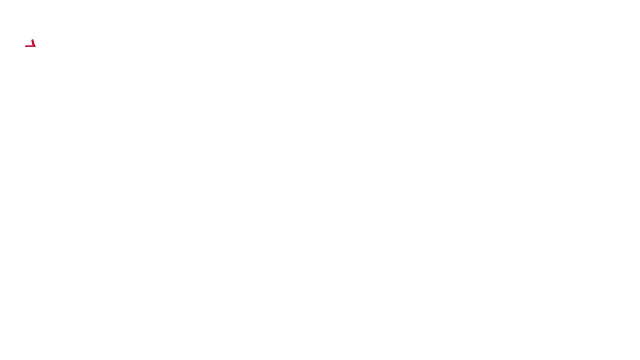 approach is used when a detailed design is available and is usually used for the budget when construction commences. So let's look at three common estimating methods used in construction. To start, we have analogous estimating. When you think analogous, think analogy, Simply meaning. 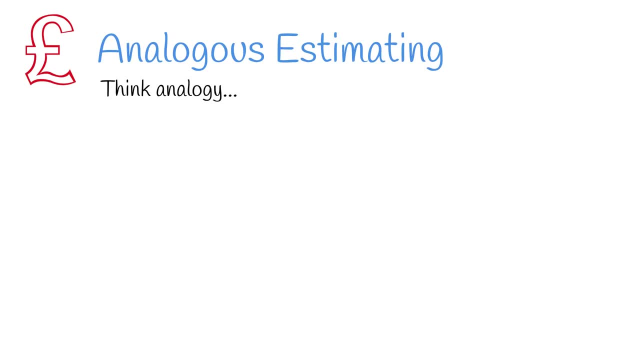 comparing one thing to another Or, in this case, one project to another. For this method, you will use historical data to find similar projects which have been carried out and use that data as a basis to form your estimate. This is often referred to as a top-down estimate. 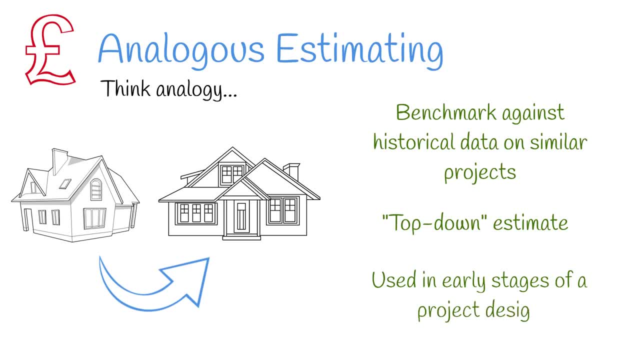 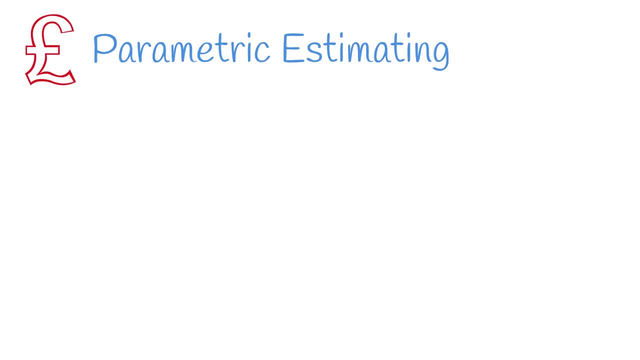 This estimation method is used when the project is in the early stages and there are limited amounts of information available. Moving on, we have parametric cost estimating. This method uses historical data to provide an estimate on what the project would cost under different conditions. 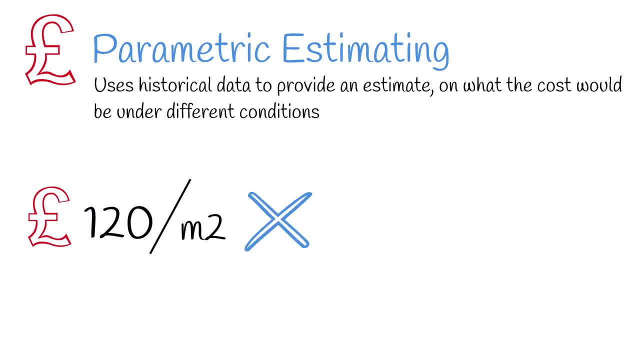 It's achieved by identifying the unit cost from past projects and scaling for the project that you're estimating, For example, square footage. This method is flexible to the level of information available. It is often considered a more accurate approach than analogous estimating.